probably more like 100 million. It used to be that there were basically only two approaches to quantum computing- Trapped ions and superconducting circuits- And those are still leading the pack. but other approaches are catching up and there's good reason to think some'll take over in the next couple of years. 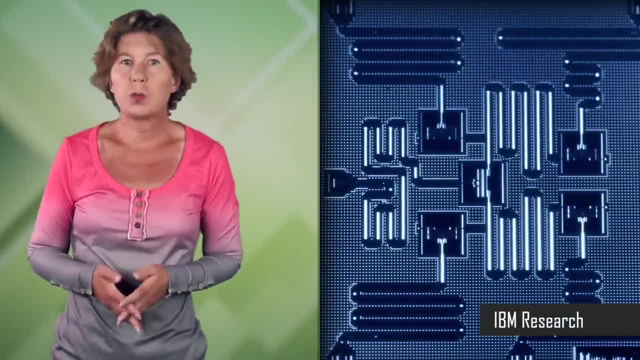 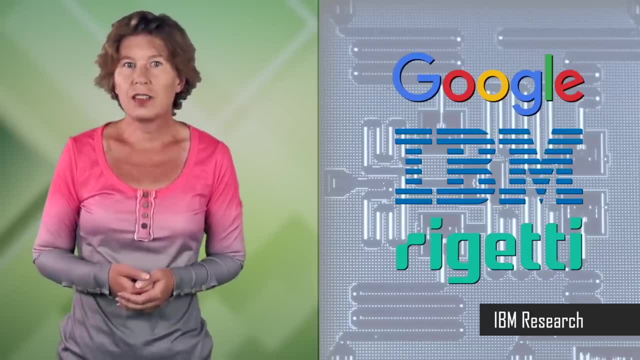 Superconducting circuits is the main approach that's been pursued by Google and IBM and Rigetti, among others. The downsides of this technology are that it's not as efficient as it used to be, But there's also a problem with these qubits, namely that the qubits need to be cooled. 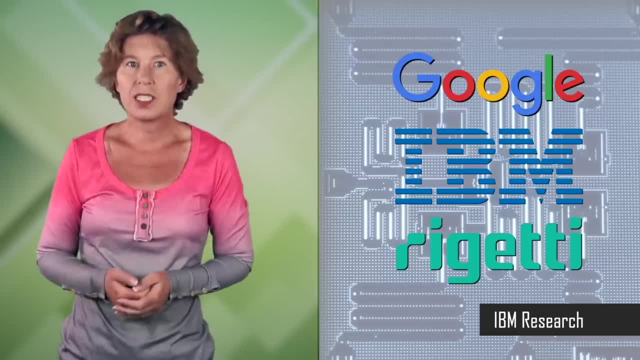 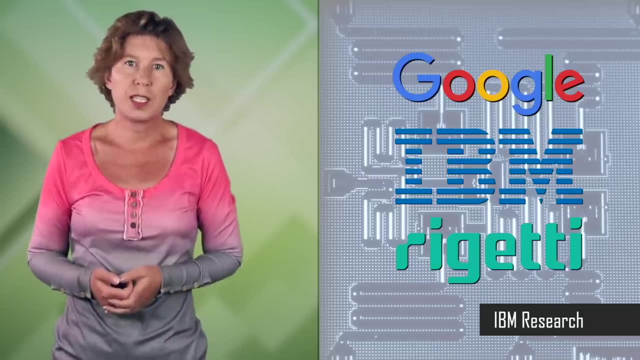 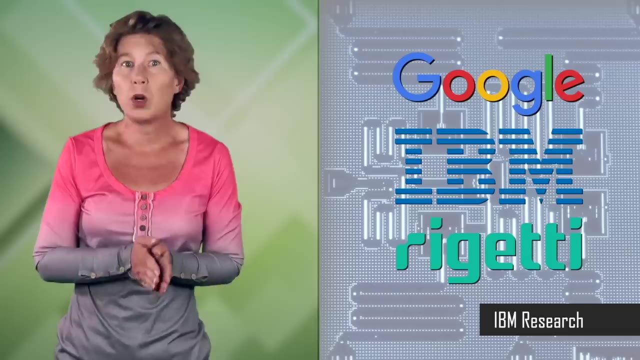 to a few milledelicons of time and that they have a coherence time that's a few tenths of microseconds on a good day. The coherence time measures how long the quantum effects last, and a few microseconds is hardly long. On the other hand, these qubits can also be operated and read out very quickly, so the 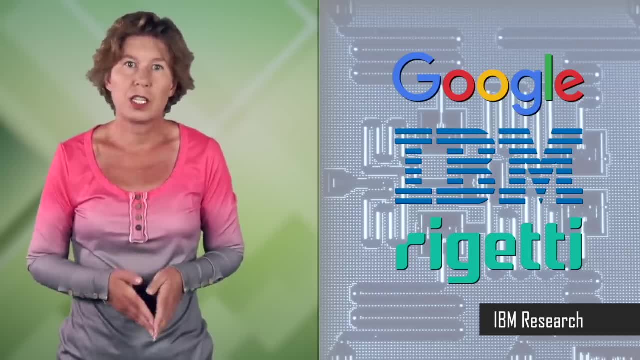 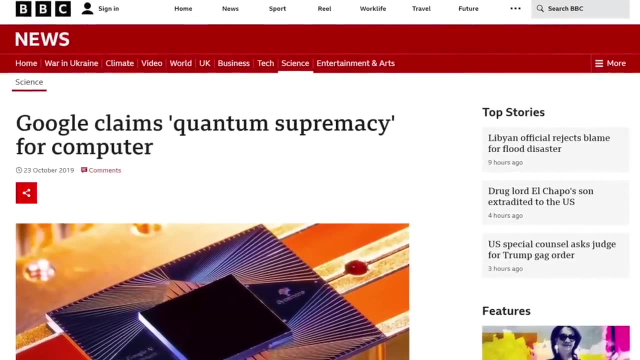 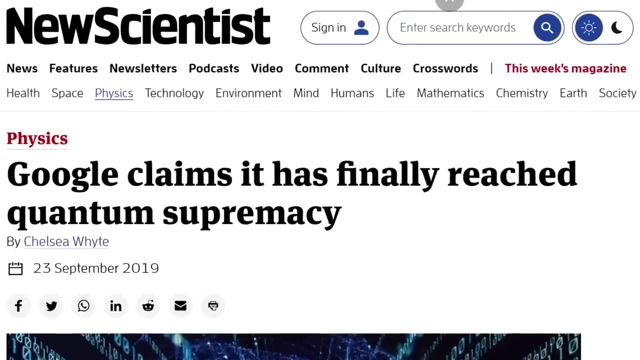 short coherence time isn't necessarily a disadvantage. Superconducting circuits are also the technology that Google needs to get used to. that Google used for the first demonstration of quantum supremacy. That's when a quantum computer performs the task faster than a conventional computer, though it's since. 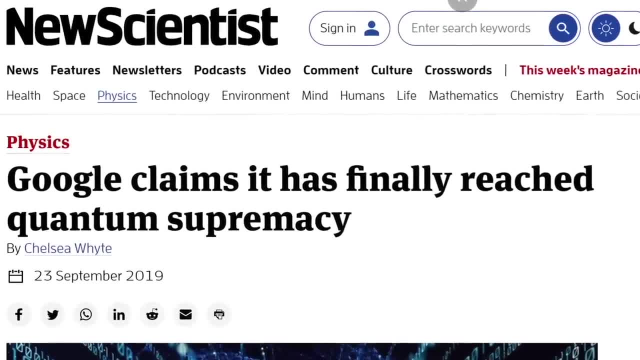 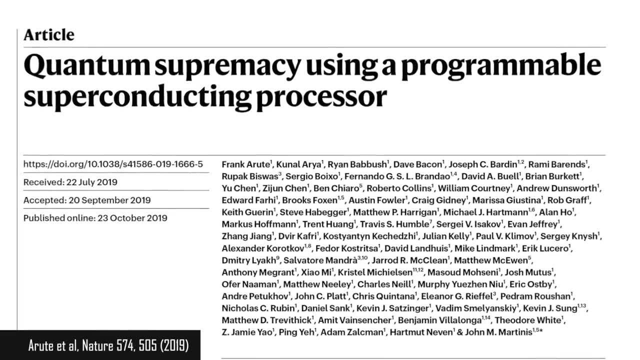 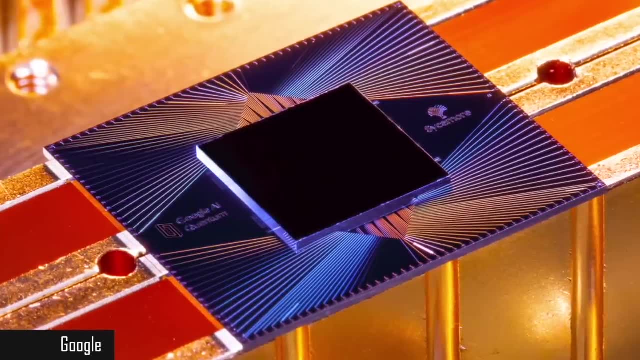 been renamed to Quantum Advantage because reasons. Google published its demonstration of quantum advantage in 2019.. They used a 53 qubit quantum computer and claimed that they succeeded in three and a half minutes with a calculation that would have taken 10,000 years. 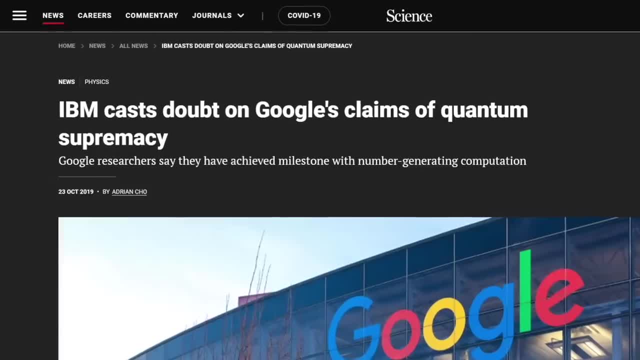 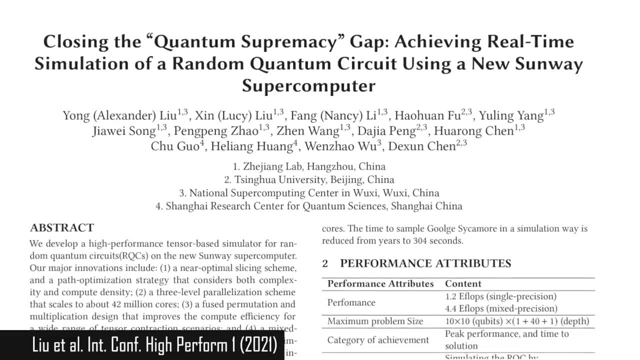 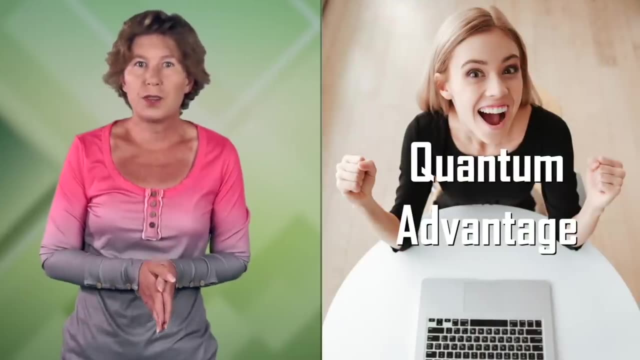 on a conventional computer. The 10,000 years claim was swiftly questioned by IBM and indeed it was later done by a Chinese group on a conventional computer in only five minutes. Quantum advantage, however, just means that the calculation was fast. It doesn't mean that it. 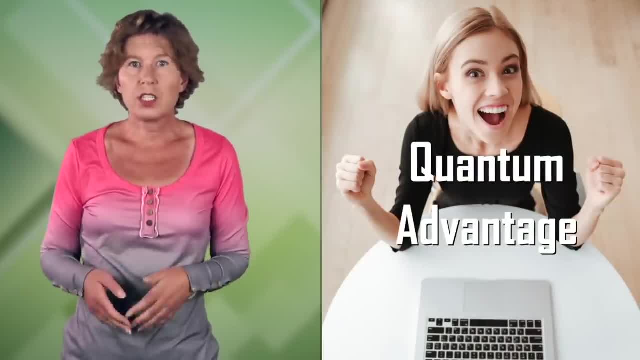 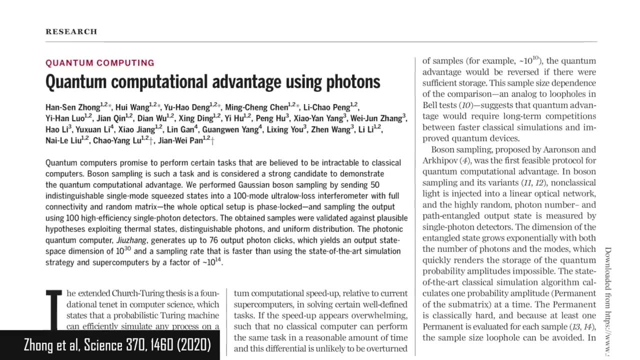 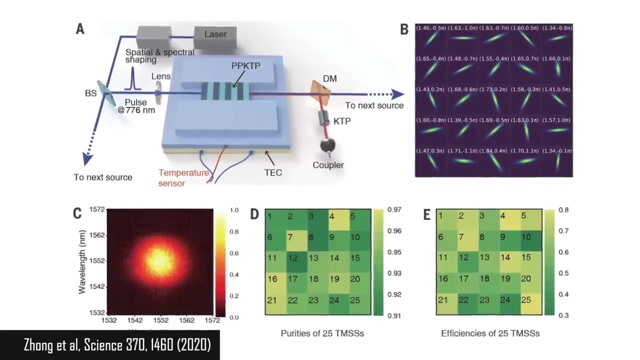 actually produced an interesting result. The calculation in question basically produced a random distribution. A similar feat was achieved by a Chinese group in 2021.. They measured coincident arrivals of 100 photons and again that produced a random distribution which is difficult to calculate by any other means. though this random distribution 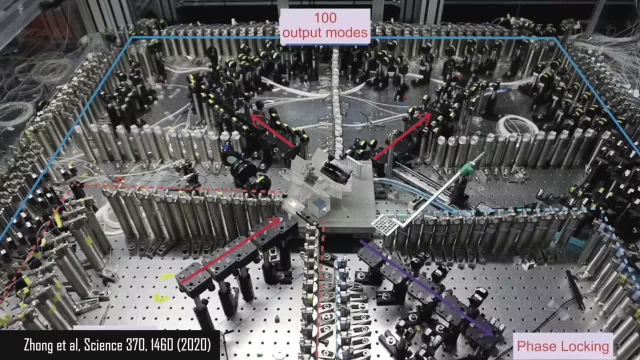 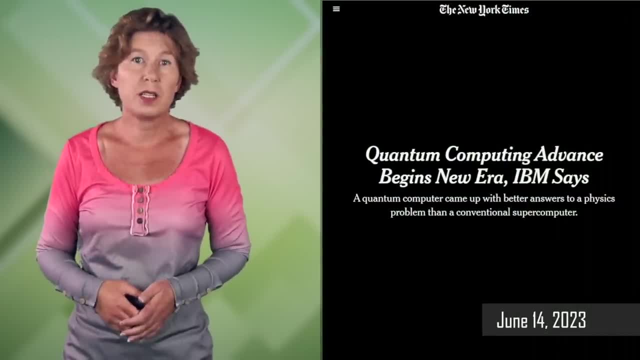 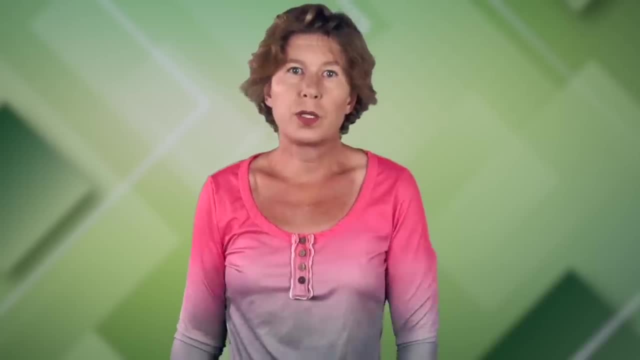 could one day have some applications. Here's a photo of their setup. Then, earlier this year, IBM made up for being beaten on quantum advantage by claiming the first demonstration of quantum utility, again with superconducting circuits. They used quantum processor with 127 qubits, called the Eagle Processor, to calculate what's called. 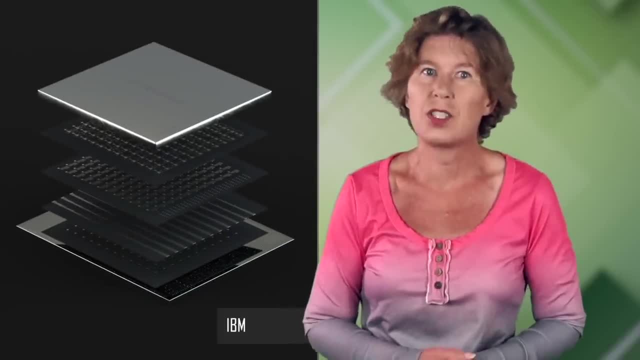 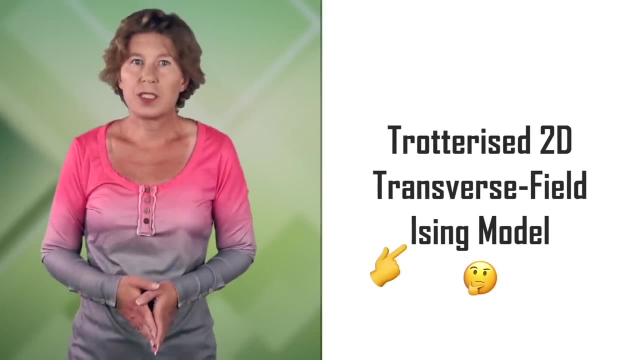 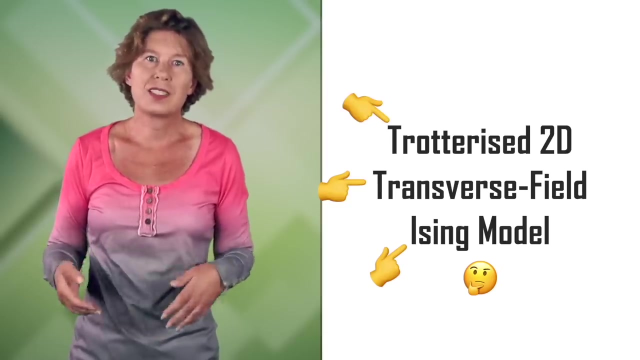 the Charterized Time Evolution of a 2D transverse field Ising model. What the heck is this? The Ising model is a model of coupled quantum spins. Transverse field means it's a complicated version of that model. That it's a Charterized Time Evolution means they used a specific method to calculate how. 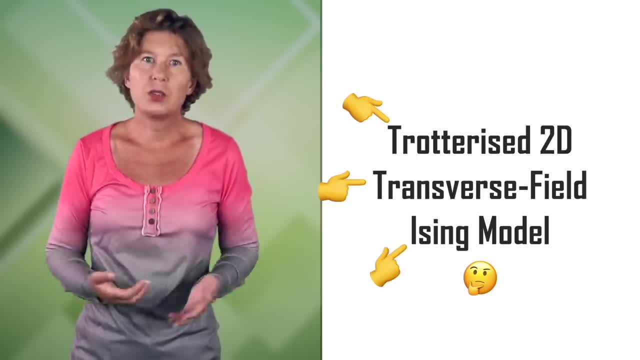 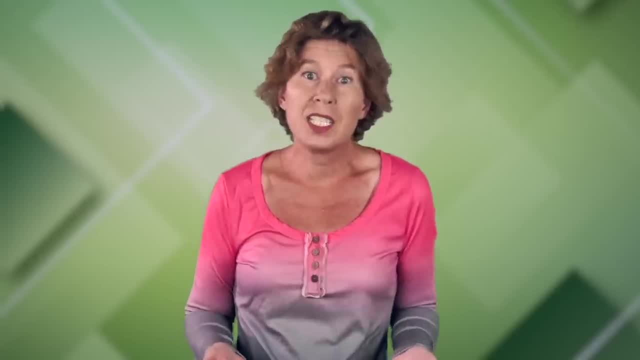 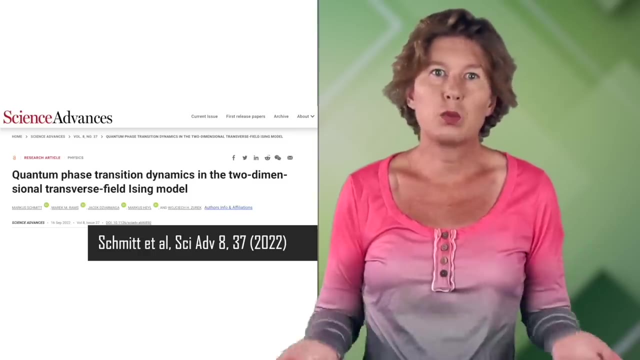 these coupled quantum spins change in time And 2D means trans-dimensional doodles. Just checking if you're listening. Now, this is a pretty amazing calculation if you're interested in the Ising model, but I think it's fair to say that this isn't exactly everyone's notion of utility. 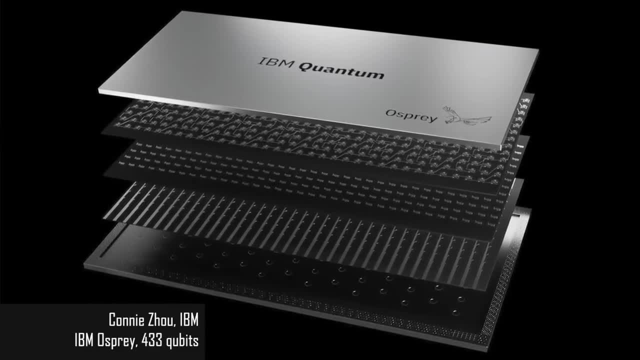 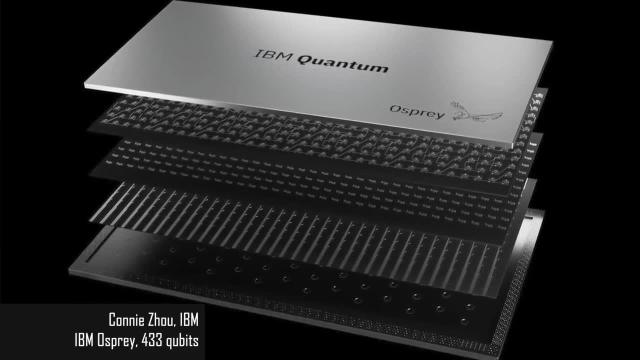 The current record for the number of physical qubits is 433, and it's the IBM Osprey chip that they're planning to make available in the cloud soon. IBM also has a roadmap according to which they want to reach more than 1,000 qubits. 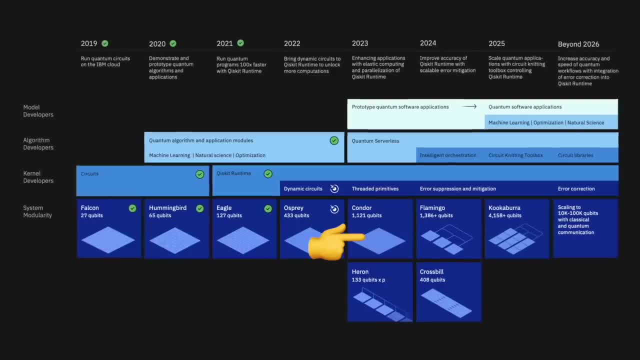 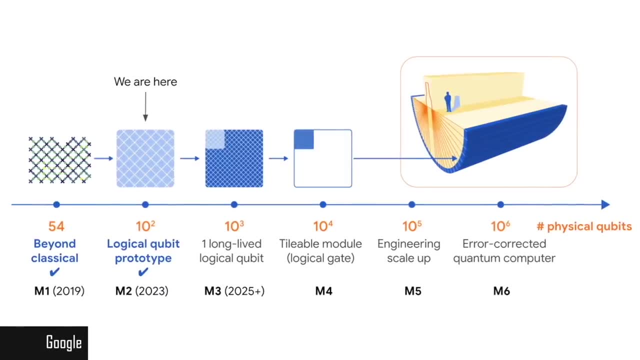 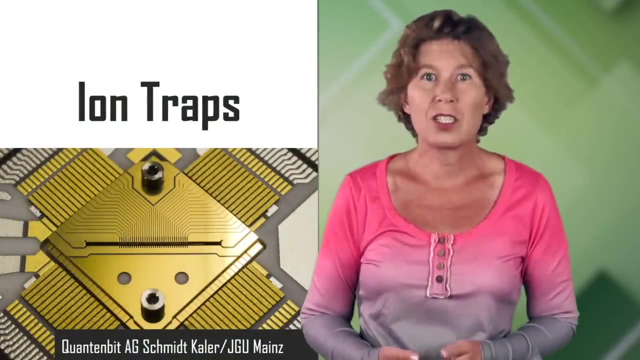 later this year. They say this'll be a modular approach which can then be scaled up to a million within ten years. Google has its own roadmap with certain milestones, but hasn't put particular dates on it. The other frontrunner has for a long time been ion traps. that has been pursued by companies. 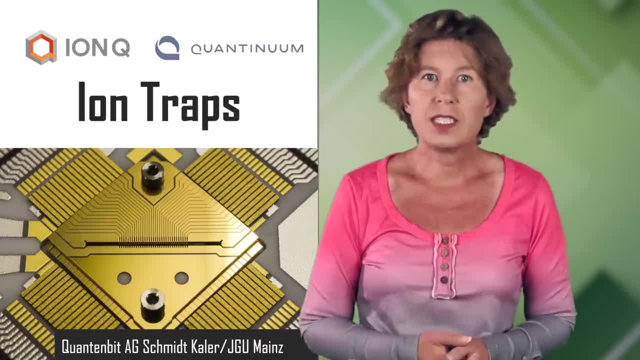 such as INQ and Quantinium. In this case, the qubits are iron And they're made of iron And they're made of iron. Iron traps are trapped by electromagnetic fields and entangled with lasers. Iron traps also have to be cooled, though not to millikelvins, but to a balmy three. 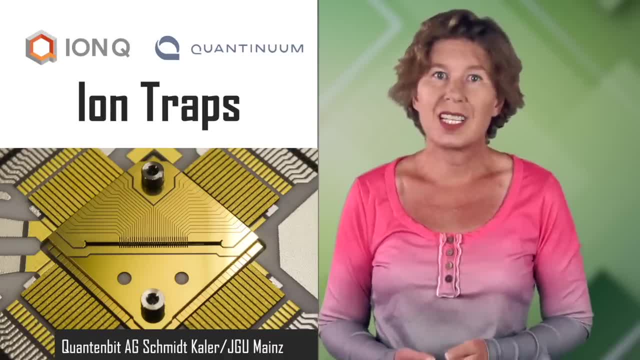 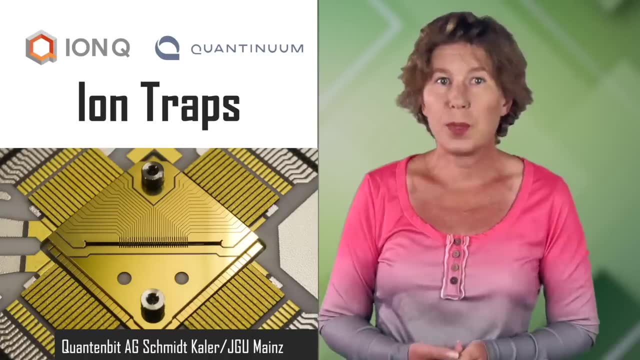 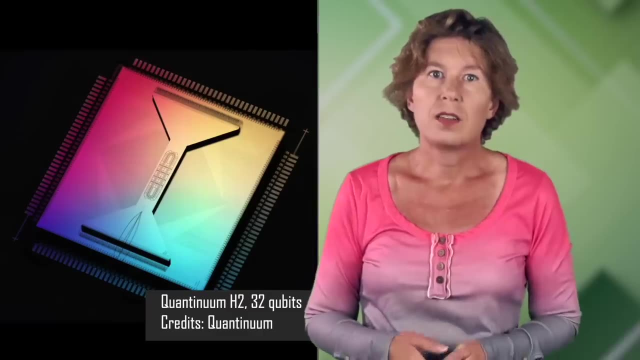 kelvins or so. Iron traps have longer coherence times than superconducting circuits, but they're also slower to operate, so it's not a priori clear which is better. In the past two years, iron traps have severely lagged behind in the number of qubits. 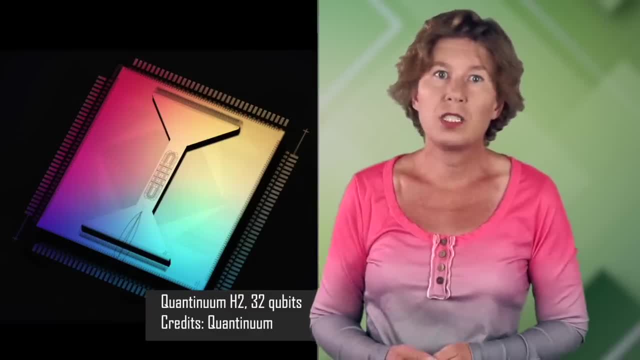 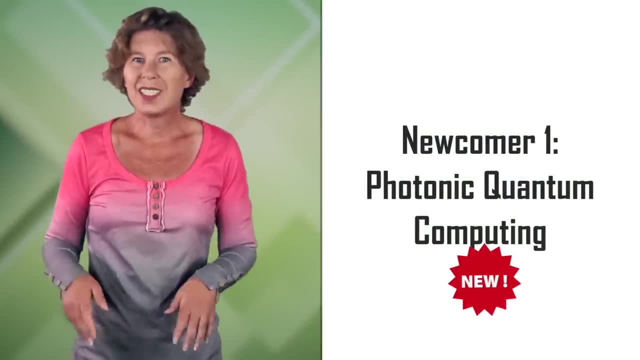 The company INQ is currently at around 4,000 qubits. The company INQ is currently at around 30, and Quantinium around the same. The first newcomer I want to mention is photonic quantum computing. When I say new, I don't mean to say that the idea is new. 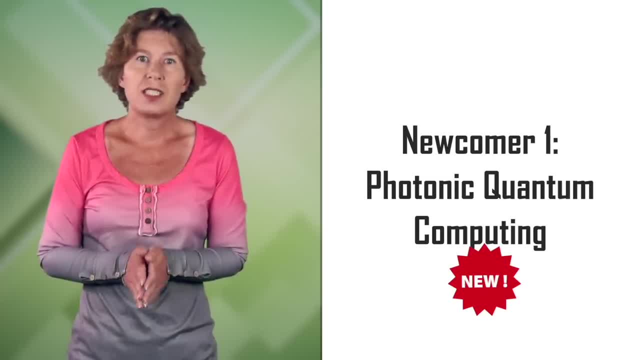 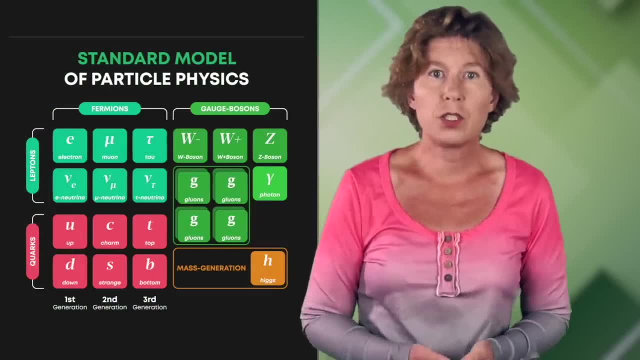 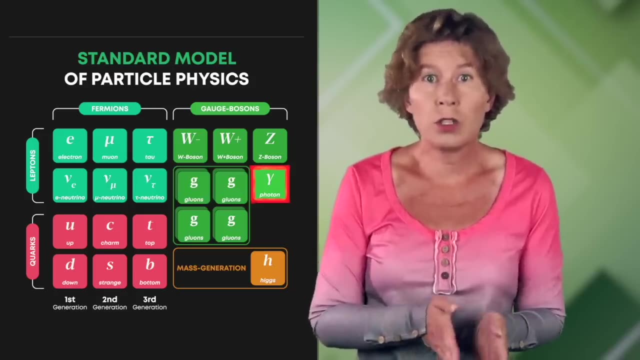 I just mean that the technology matured a lot recently and they have something to show for it. Photonic quantum computing, as the name suggests, uses photons as qubits. In the simplest case, the two qubit states are just whether the photon is there or not. there. The good thing about photons is that you can use them at room temperature, though you still need to cool the detectors down, because otherwise you can't find the single photons in the noise. The challenge for photonic quantum computing is: well, first you need to have reliable 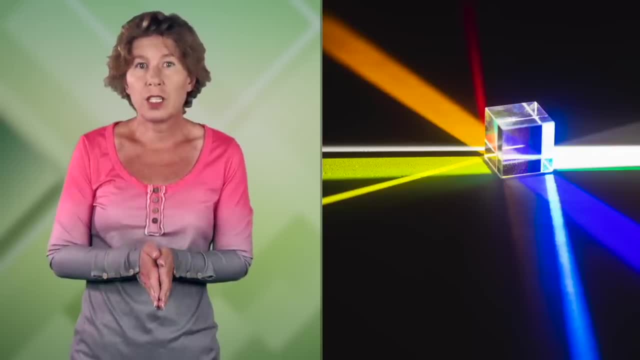 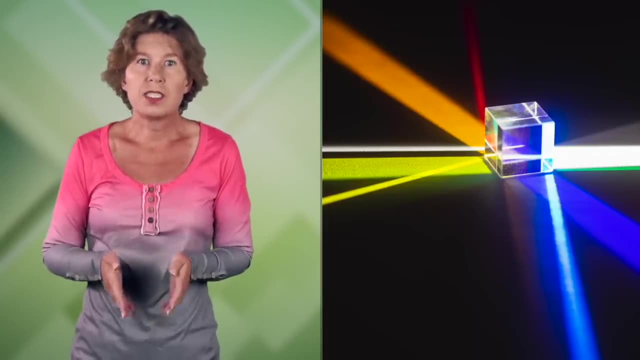 sources for single photons. and then you have to shrink down all the elements that you normally have on an optical table and put them on chips. This isn't all that easy. Photons are the qubits. Photons are the quanta of light, so they move well at the speed of light. They don't just sit around and wait for you to get things done. You have to shrink all these elements down so that you can scale the device up. Remember the setup from the Chinese group. This is for 100 photons. Let's say it's about one or two square meters. and now scale this up to a million. 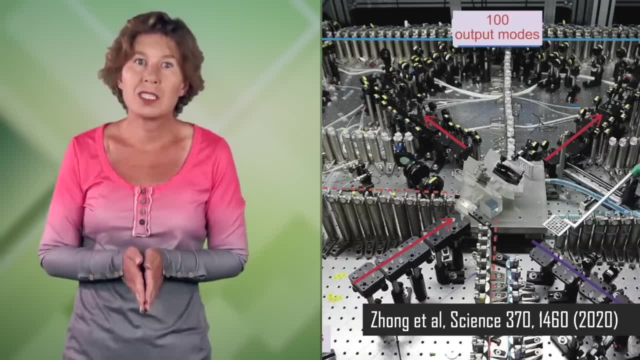 photons, That'd bring us to more than 10,000 square meters, which is about the size of a computer, And that's it. Photons are the quanta of light, so they move well at the speed of light. You have to shrink down all these elements down so that you can scale the device up. 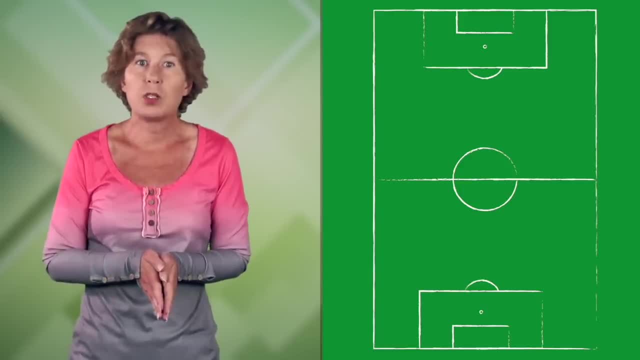 Let's say it's about one or two square meters and now scale this up to a million photons, That'd bring us to more than 10,000 square meters, which is about the size of a football field. It's kind of hard to control perturbations of a device that large, so maybe you begin. 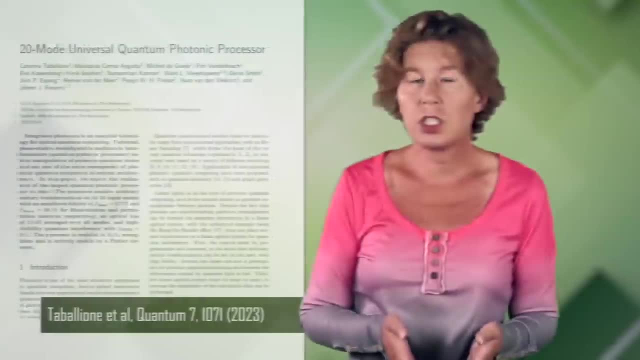 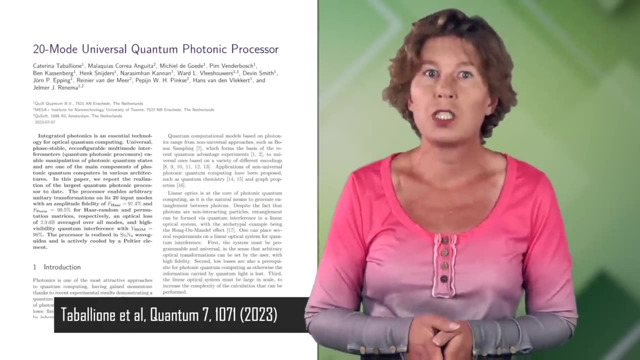 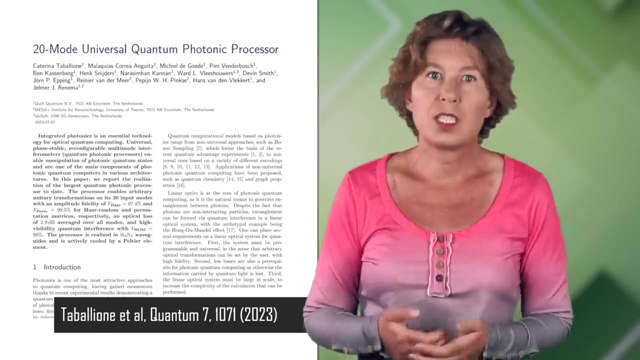 to see the problem here, But scientists have managed to build chips that can perform many of those operations off an optical table, and some basic photonic quantum computing chips now exist. For example, a Dutch group related to the start-up, QuixQuantum, recently presented a 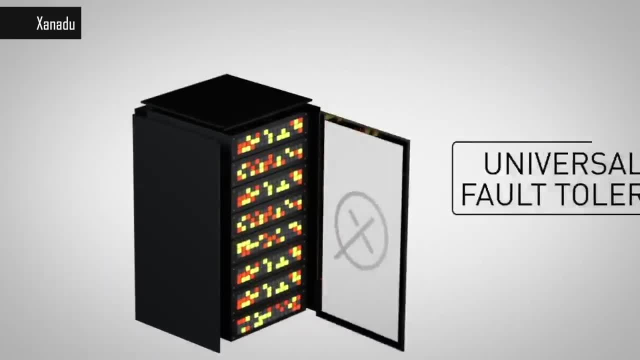 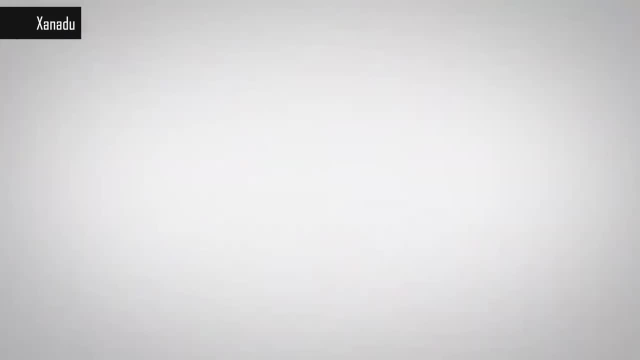 20-qubit photonic chip. In 2022,, the Canadian company QuixQuantum will be able to build a 20-qubit photonic chip. The company Xanadu even put forward a 216-qubit photonic quantum computing chip, which they 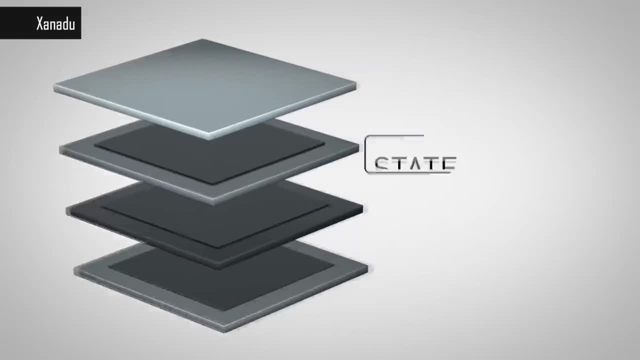 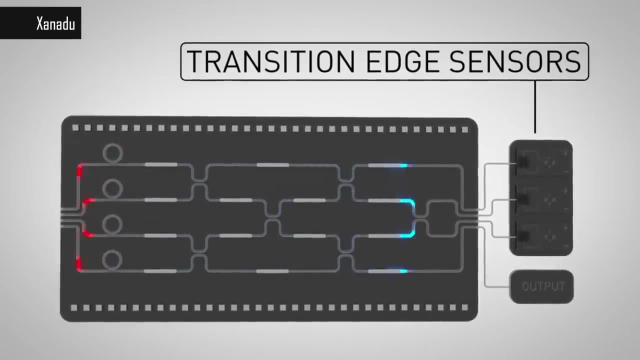 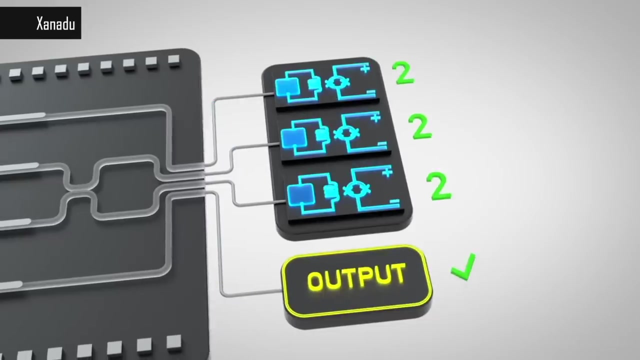 called Borealis. They are using a technology made of four layers to encode the quantum state and then operate on it. Their qubits are squeezed states of photons that are basically optimized states, Though they stress that, by the nature of their states, their system is not equivalent to. 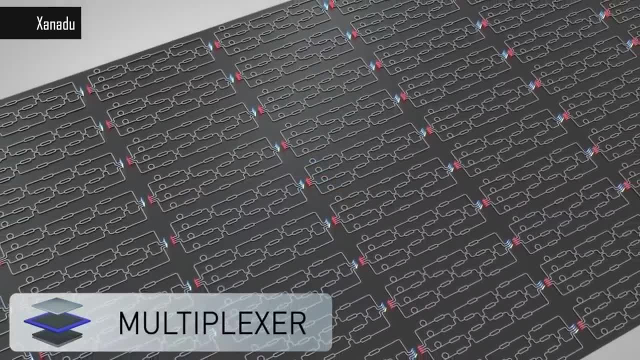 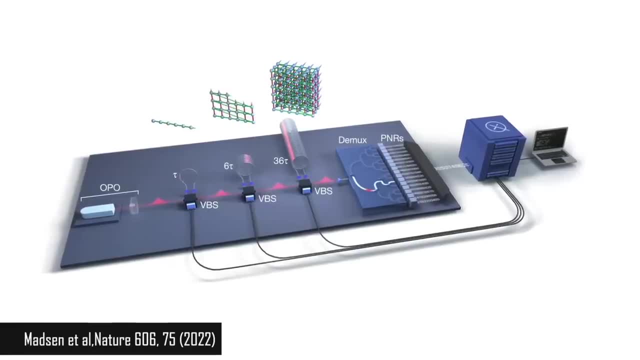 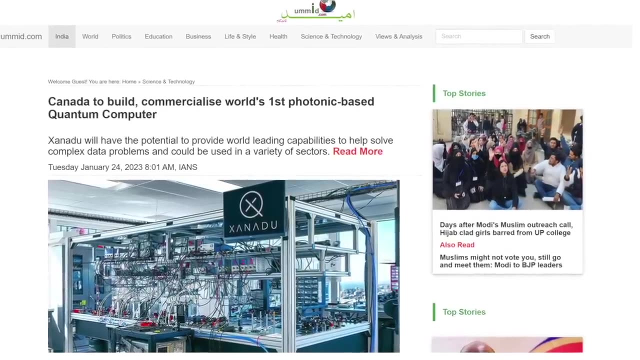 a universal 216-qubit processor, as it can only do certain tasks. In the meantime they have published a paper in Nature demonstrating quantum advantage also for a sampling method. Earlier this year the Canadian government invested 40 million Canadian dollars into the company. 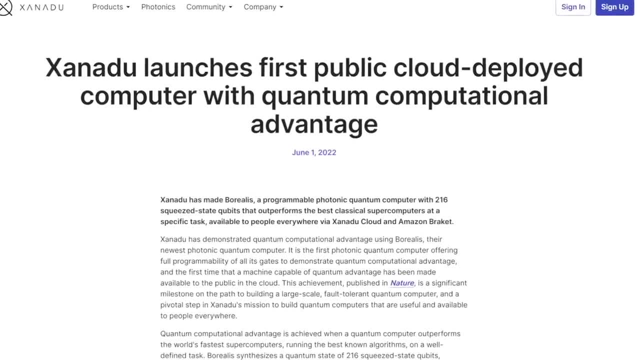 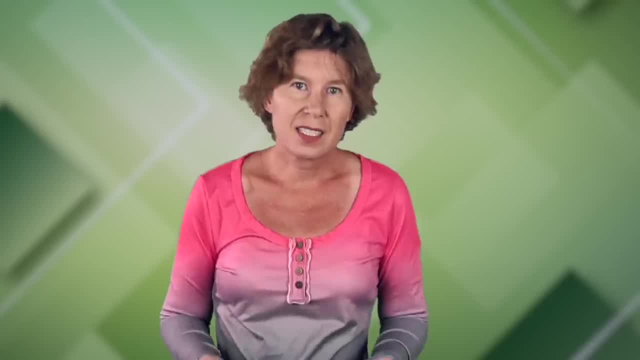 Xanadu says that their technology can be scaled up to a million qubits. at least Xanadu has made Borealis available for use for everyone over the cloud. Yes, this is well behind IBM's 400, or maybe soon 1000,, but this delay might not matter. 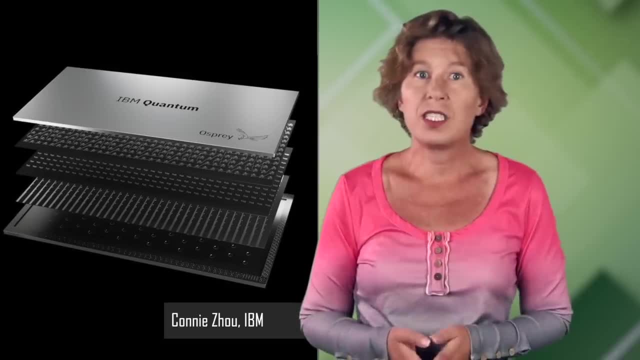 all that much in the end. I hope you've enjoyed this video and, if you did, please hit the subscribe button and the bell to not miss any future videos. Thank you for watching. See you in the next one. Bye. This is certainly also what the company PsyQuantum thinks. 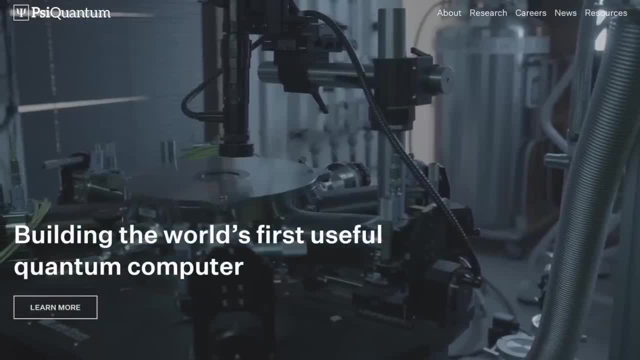 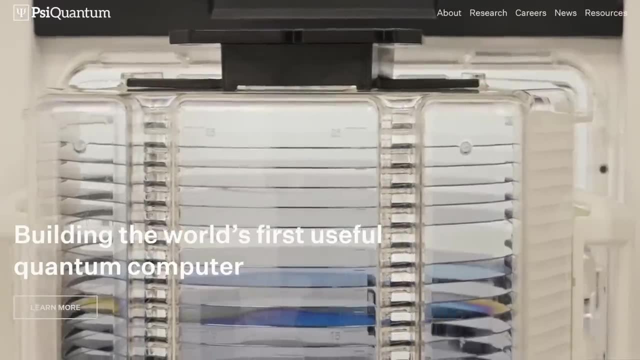 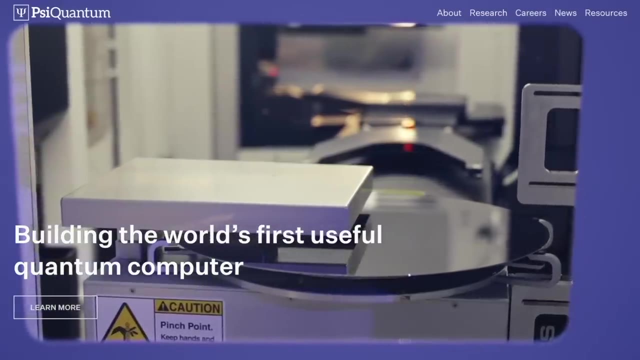 The company has partnered with Global Foundries, a leading semiconductor producer, to manufacture chips for photonic quantum computing en masse. They say that they want to have the facility for chip fabrication in place by the middle of the decade and then have their million-qubit quantum computers shortly after that. 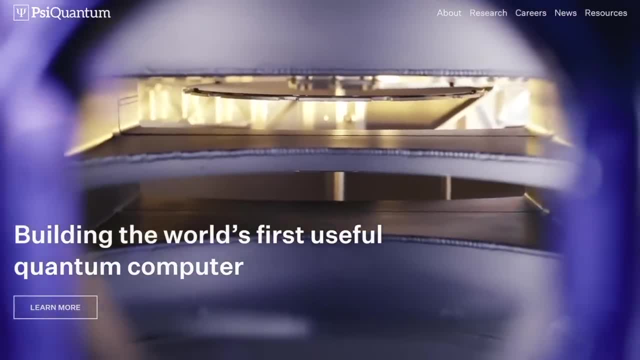 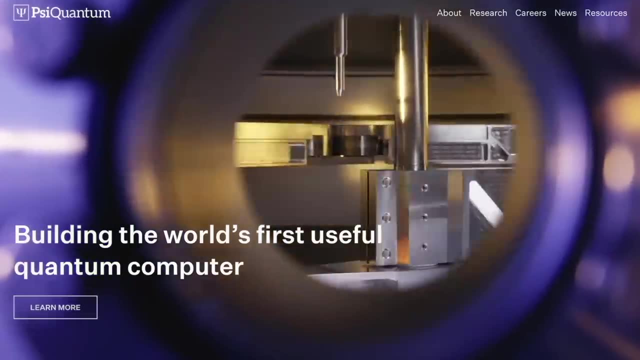 PsyQuantum has been extremely quiet on their technology, so it's hard to say how far along they really are. That you can't really tell what they're doing could be a good sign, because they might be very worried that they're getting scooped. 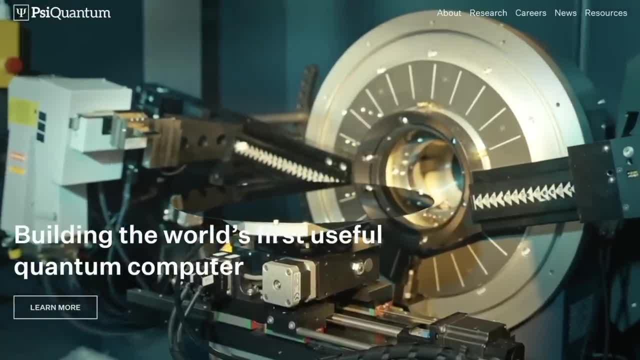 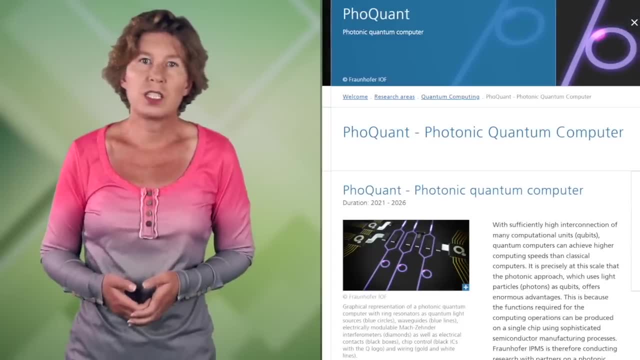 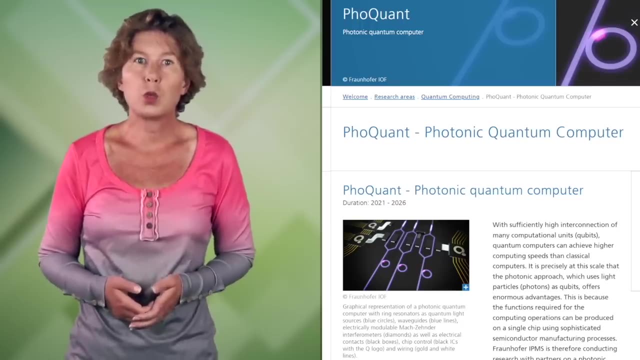 or it might be a bad sign, because it's really just hot air. The Germans too are interested in photonic quantum computing. A public-private partnership of 14 organizations is working on a project called FocQuant, which aims to develop a photonic quantum computer with up to 100 qubits by 2026.. 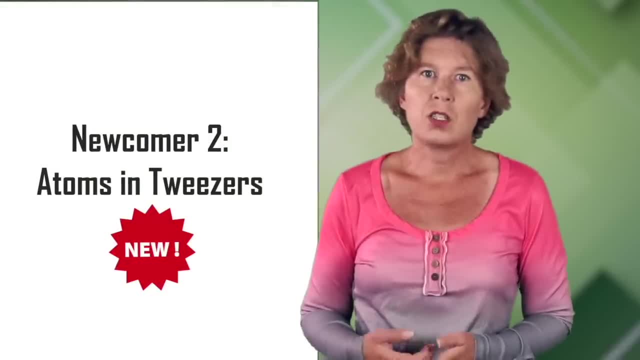 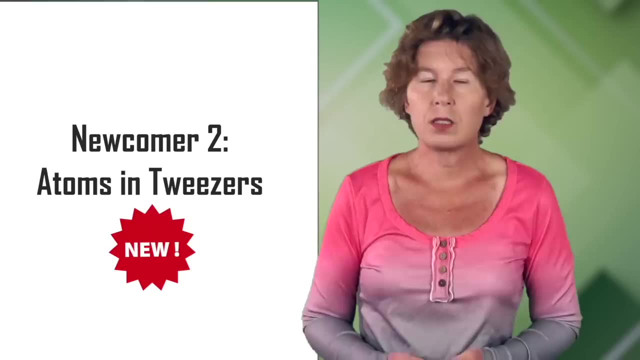 Newcomer number two are atoms in tweezers. Not exactly the kind of tweezers you pluck your eyebrows with, but tweezers made of light, so-called optical tweezers. Atoms in tweezers are a variation of the idea of ion traps. 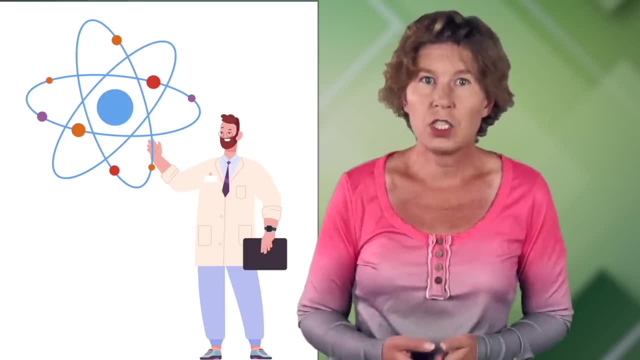 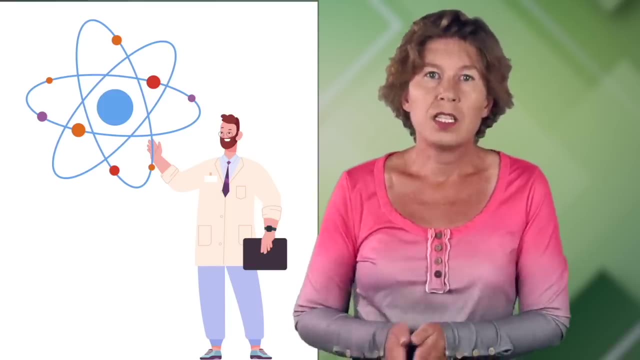 Ions are atoms that are missing some electrons, so they're negatively charged. On the one hand that's good, because if they're charged they're easier to trap. On the other hand it's bad, because they all repel each other. 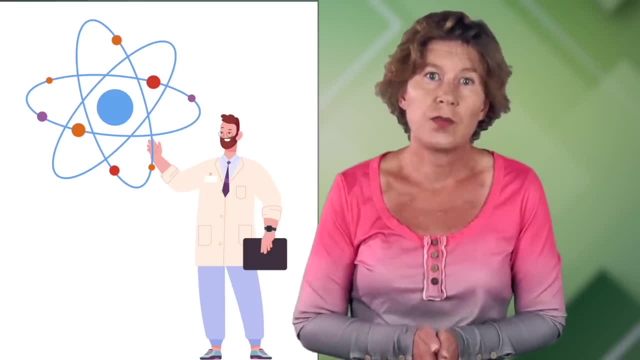 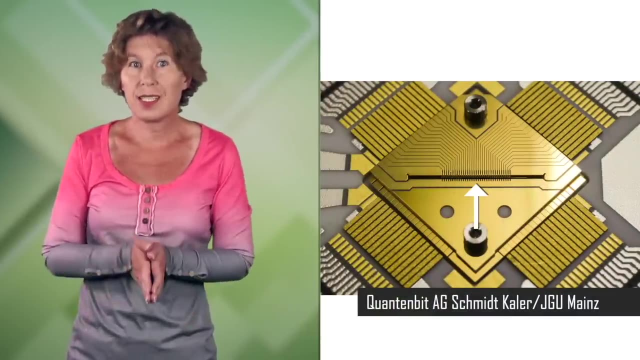 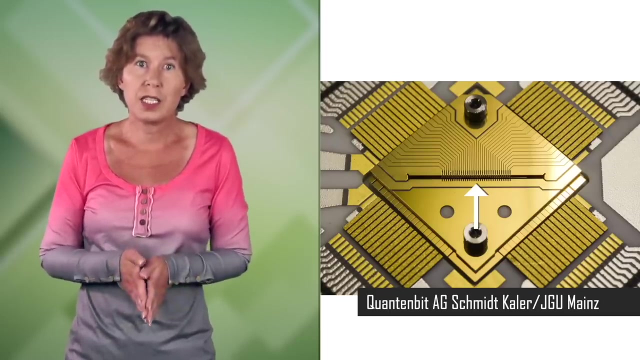 which makes for awkwardly unstable configurations. In the currently used ion traps the ions all sit in a row. It's called a linear trap, and it's convenient because the ions in a linear trap are reasonably easy to handle. You can link several of those traps with each other and that's been done. 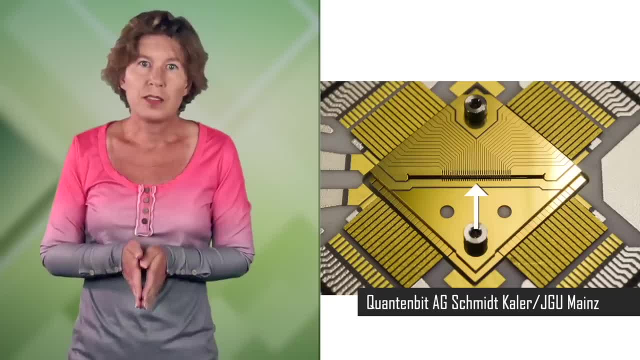 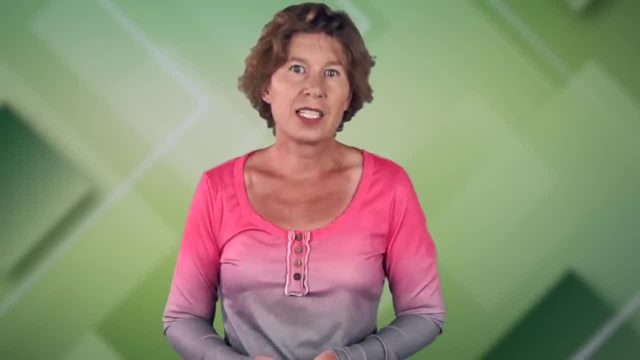 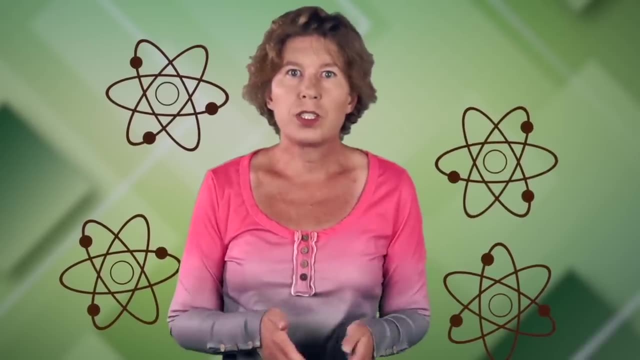 but if you want to keep on lining them up forever, that doesn't scale very well. if you also want them to all interact, If you instead take neutral atoms, that makes it easier to build three-dimensional configurations and that scales better. This is what you do with the optical tweezers. 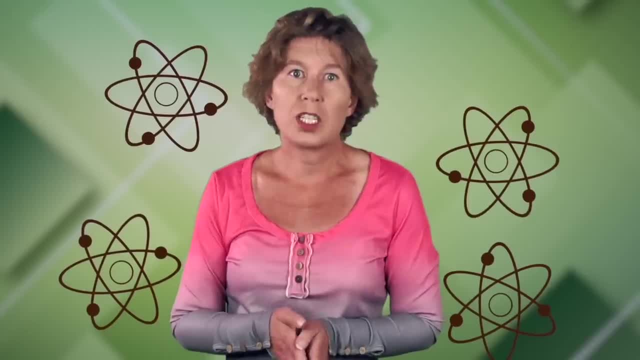 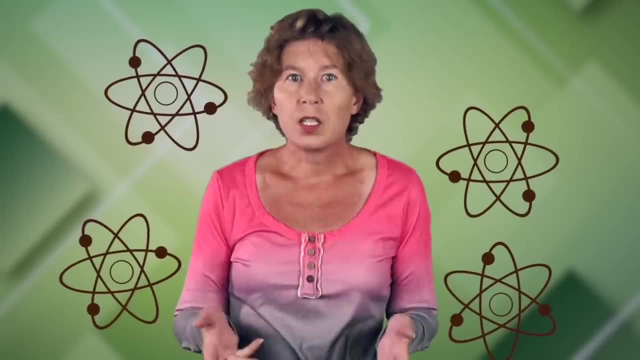 They're weak, so they don't work well on charged things like those ions, but they're big at the moment because they're more scalable. You then need some way to encode qubits in the atoms, and there are several ways to do that. 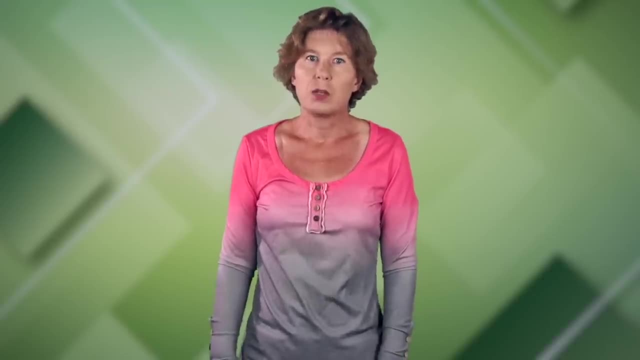 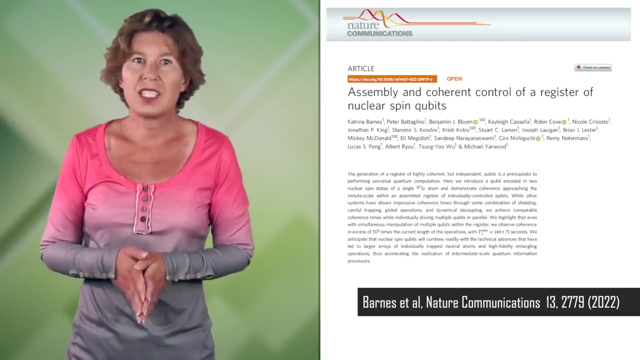 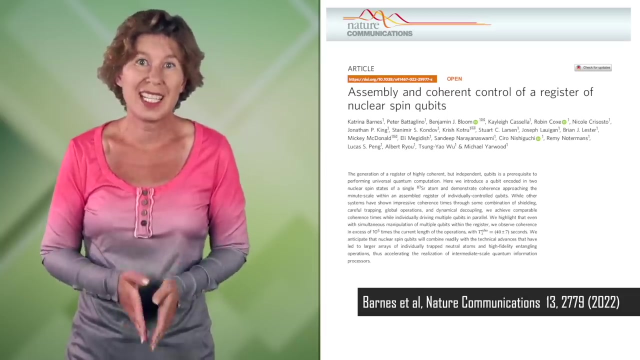 You can do it, for example, with nuclear spin states, which is what the California-based start-up Atom Computing is doing. They are using two different spin states of strontium-87 atoms. In a paper last year they said they observed a coherence time longer than 20 seconds. 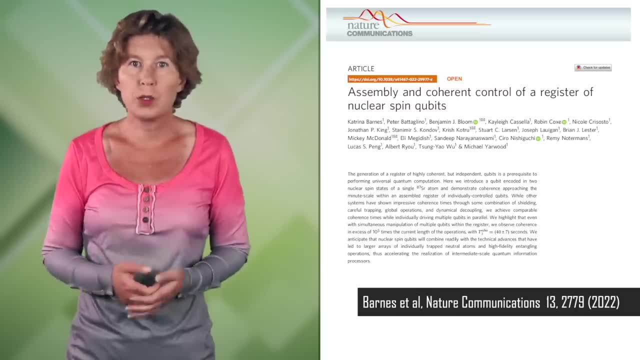 I can report from my own experience that, when it comes to quantum computing, staying coherent for more than 20 seconds is a remarkable success indeed, The company says that to date they can work with about 100 qubits, which is pretty good. There's also the company ColdQuanta that said until 2022, they want to have 100 qubits in the form of cold atoms, But 2022 came and went and I saw no press release of such a device. They published a paper in which they report successfully computing with 6 qubits. The website now says they want to have 1000 qubits by 2024.. It's a lot of work, And the first one is Pascal, and a lot of research institutions are looking into it as well. The third newcomer is topological quantum computing. 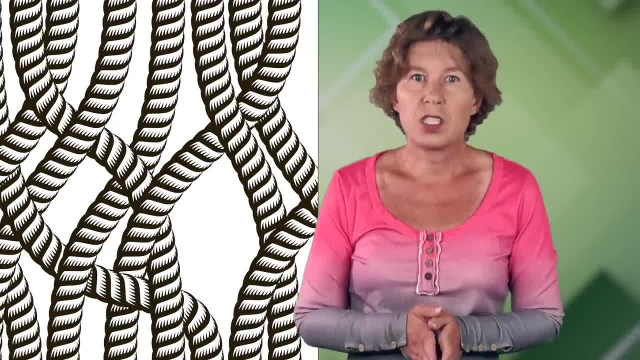 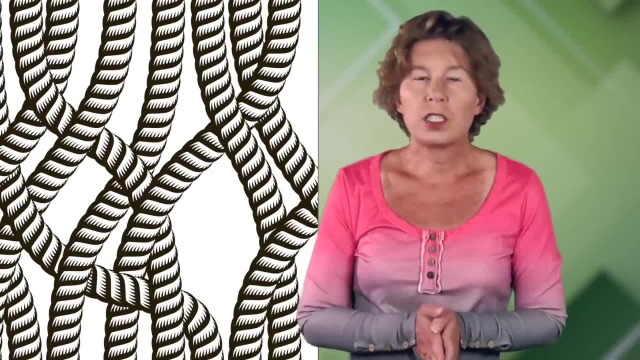 Topological quantum computing is a somewhat different idea from all the rest, in that the term doesn't refer to the physical basis of the qubit, but rather the type. A topological qubit can be realized in many different ways. The relevant point is that it's a collective excitation in some kind of media. 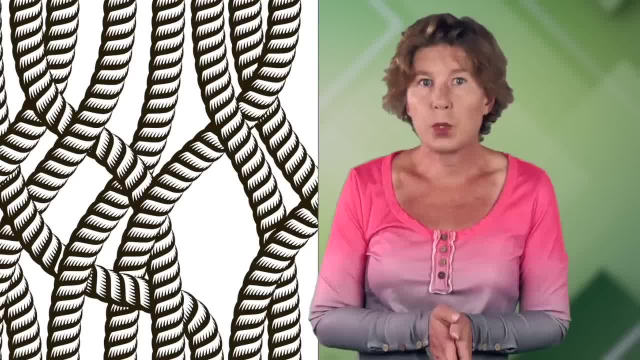 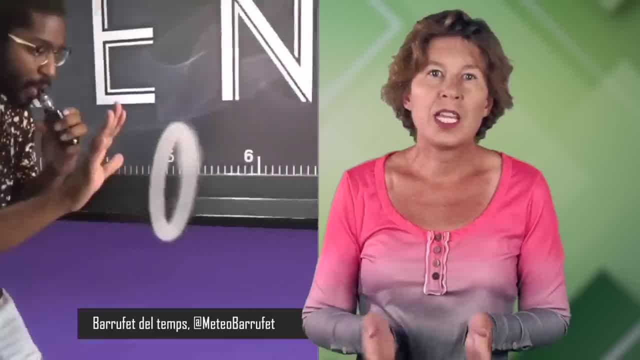 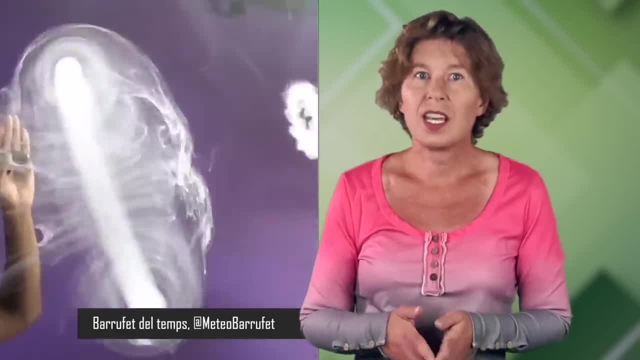 The quantum properties are protected because they're a conserved quantity, a topological property. They're like smoke rings: made of smaller particles but have a shape that they want to keep. This makes them robust to noise and that's why they're interesting. Topological quantum computing was basically 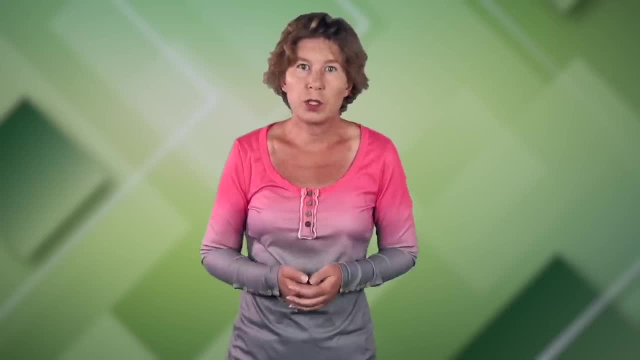 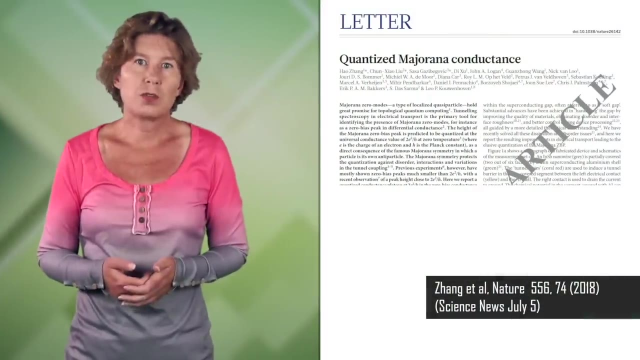 only pursued by Microsoft, or so everyone thought, and that wasn't going all that well. A paper published in 2018 in Nature by a Microsoft-led team claimed to have found evidence of Majorana modes, which are a type of topological quantum state. 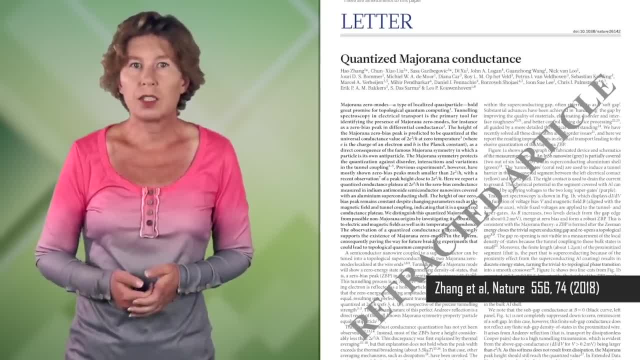 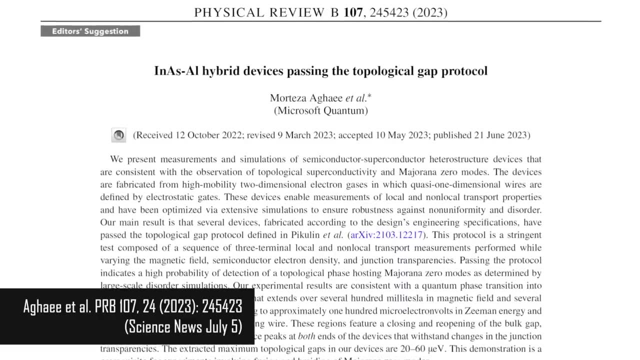 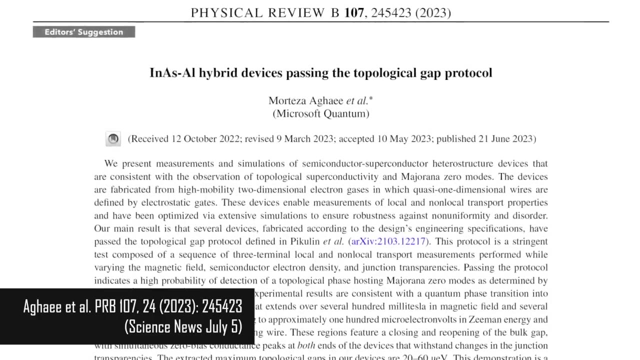 However, the paper was retracted in 2021 after the authors admitted to having made mistakes in their data analysis and presentation. But in June this year, another group at Microsoft put out a new paper in which they say again that they've successfully created such Majorana modes. They used a thin 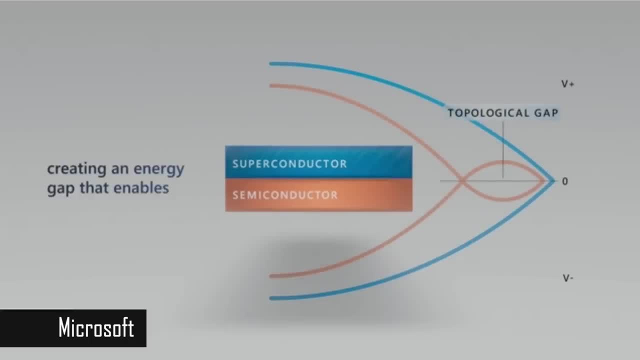 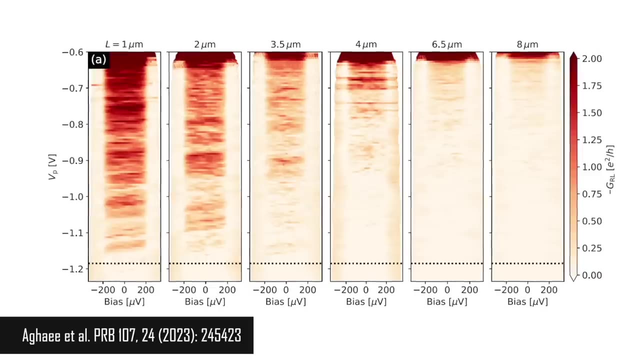 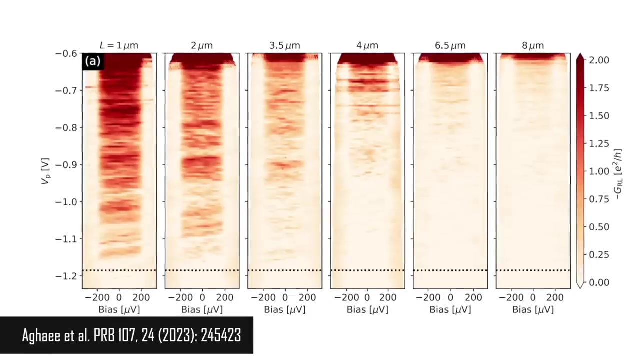 superconducting wire coupled to superconducting aluminium and claim they have convincing evidence for Majorana modes on the endpoints of the wire. This device still needs to be cooled to 20 millikelvin or so, but if they were right, it would be much easier to scale up quantum. 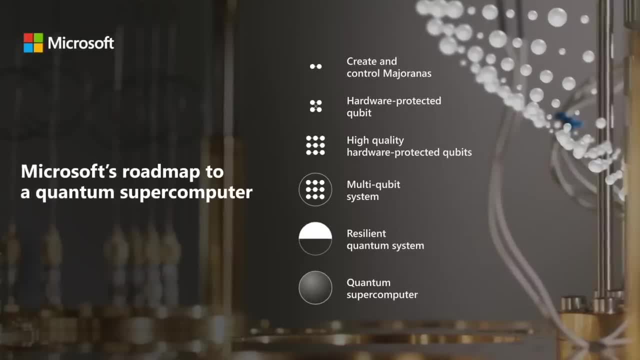 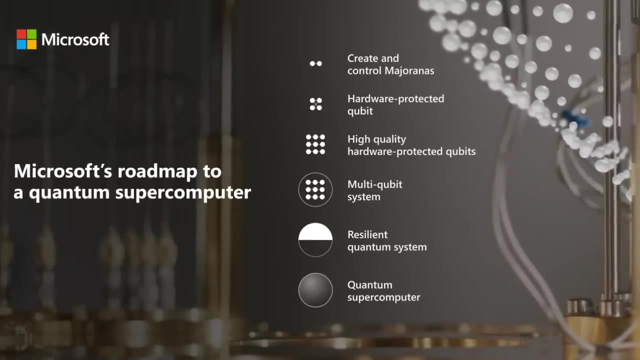 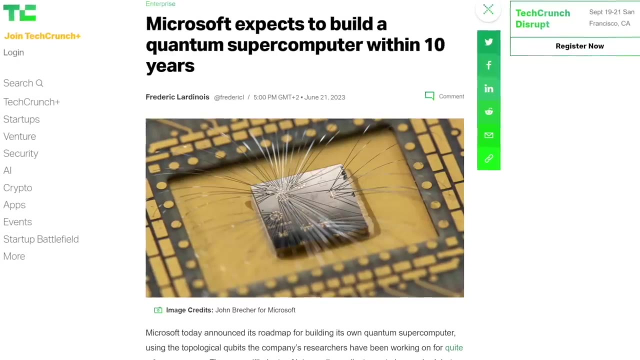 computers. Microsoft also has a roadmap for quantum computing. It makes no specific statements about how long it's going to take, but in an interview with TechCrunch, Krista Svore, who leads the quantum research group at Microsoft, said that it'd take less than 10 years. 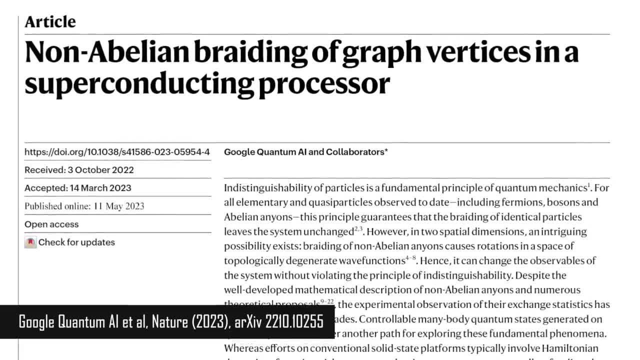 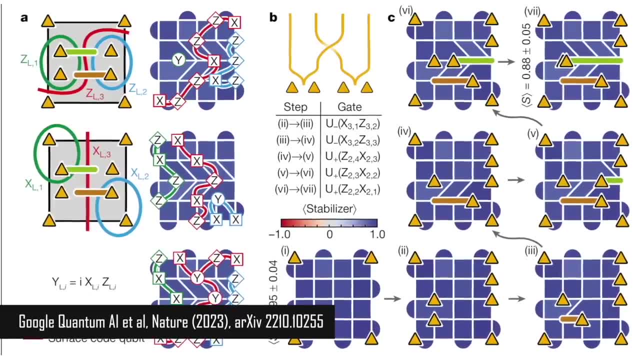 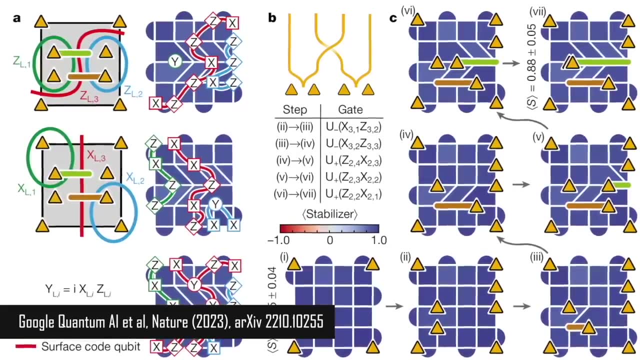 The maybe most surprising development has, however, been that suddenly, several other companies are interested in topological quantum computing as well. In late 2022, Google's Quantum AI group announced that they, too, had successfully created a different type of topological quantum states- the nonhabilions They said they had. 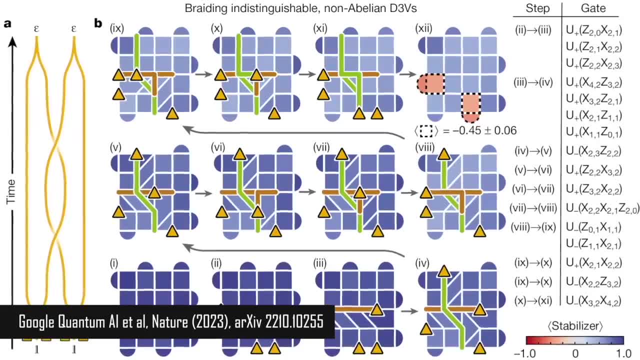 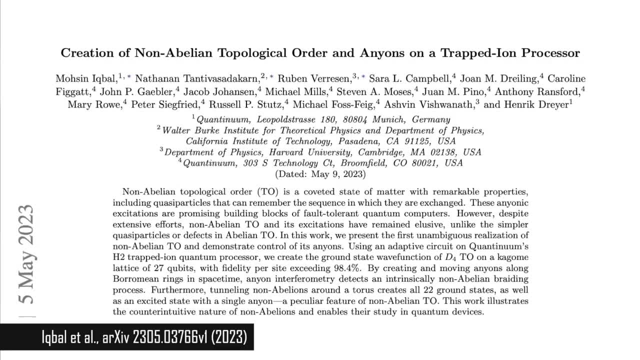 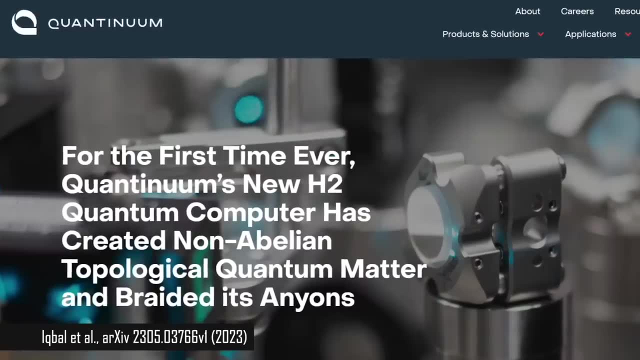 made that work on a superconducting processor and they also encoded information in them. And in May this year a group of German and American physicists, together with the quantum computing startup, Quantinium, have created another type of topological quantum state. 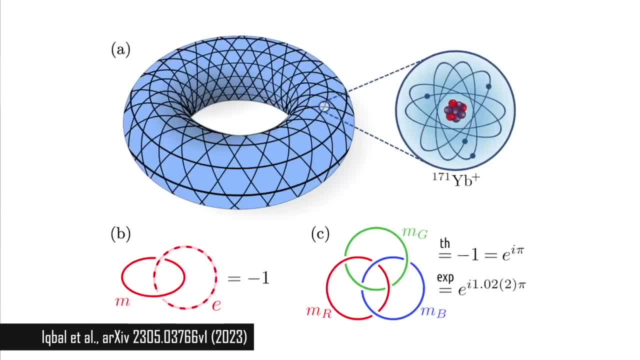 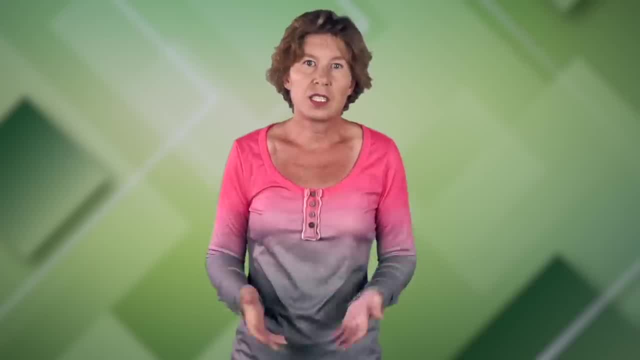 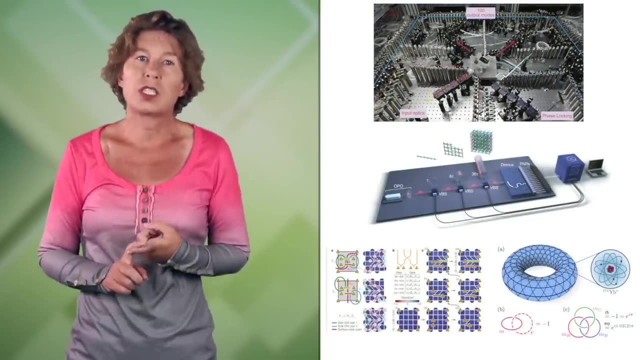 similar to that of the Google group. They realised these states on an iron trap with 27 qubits and they also managed to entangle them. In summary, a lot has happened in quantum computing in the past two years, with two strong newcomers. 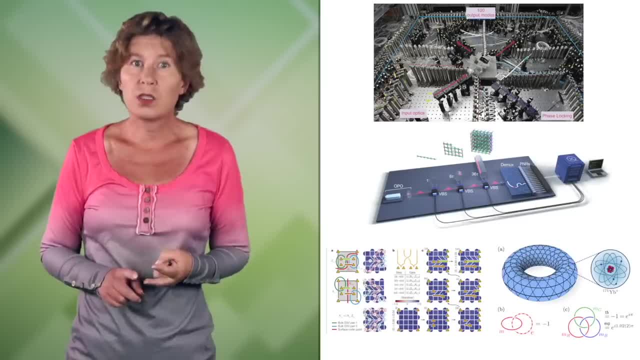 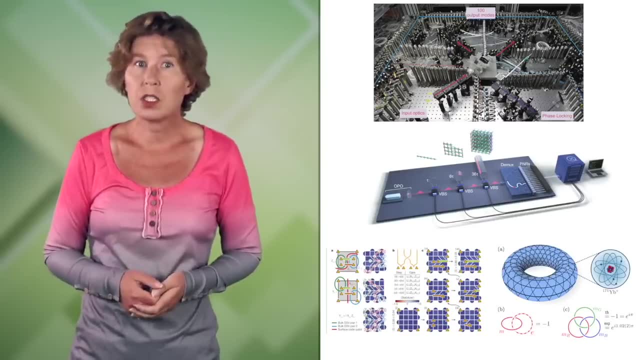 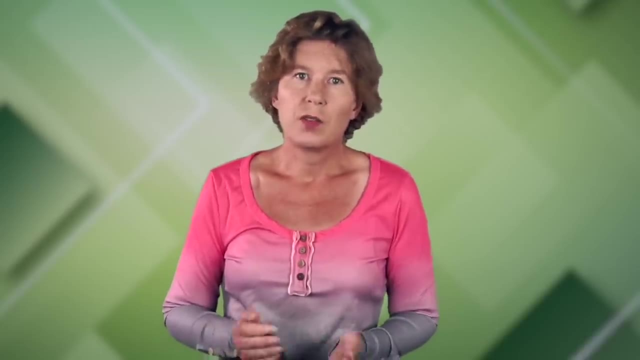 photonics and optical tweezers and dark holes catching up, that's topological qubits. I quite frequently talk about this in my weekly science news, so rest assured I'll keep you up to date. Okay, I admit that I didn't actually explain how quantum computers work. That's because I 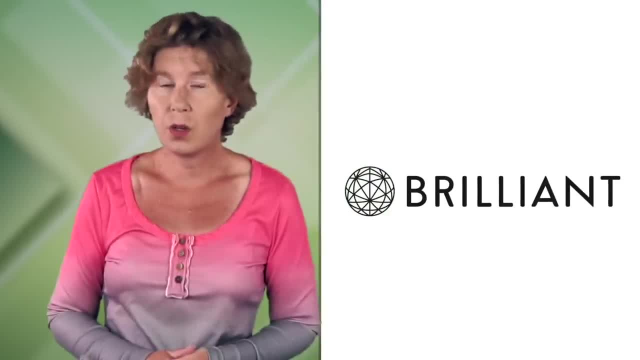 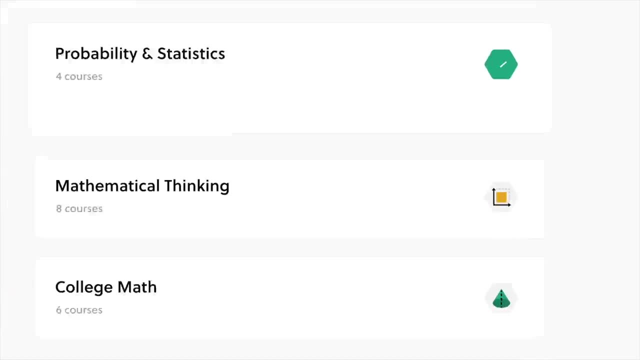 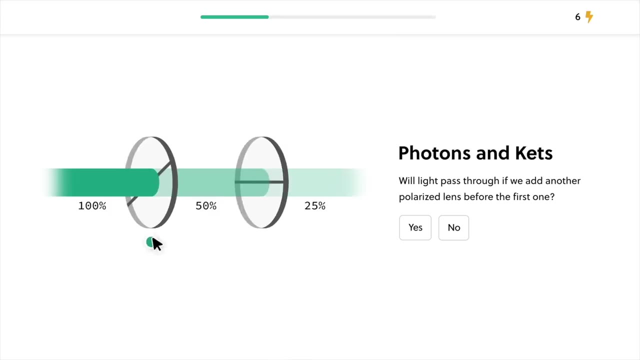 know a free and easy way you can learn this at Brilliantorg. Brilliantorg. Brilliantorg offers courses on a large variety of topics in science and mathematics and they're adding new content each month. All their courses come with interactive visualisations and follow-up questions. They have a great course on quantum computing that'll really 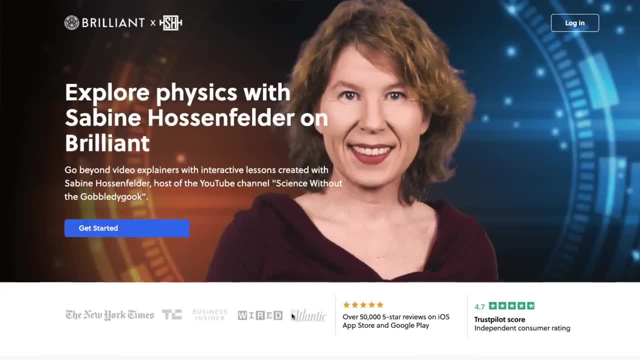 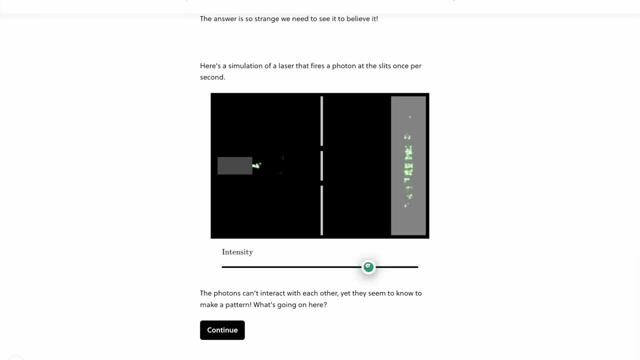 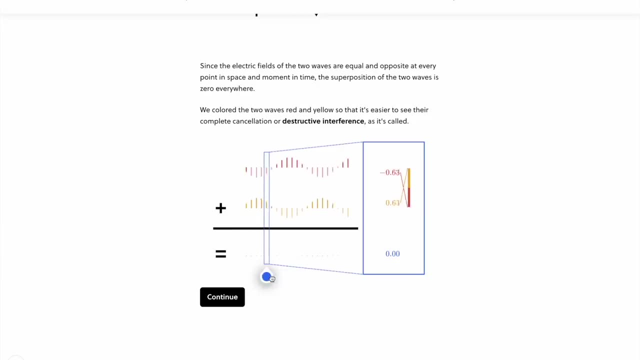 give you a feeling for what is going on. If you first need a little more background on quantum mechanics, check out my own course on Brilliant. It's a beginner's course and covers topics such as interference, superposition and entanglement, the uncertainty principle and Bell's theorem. Brilliant also covers a